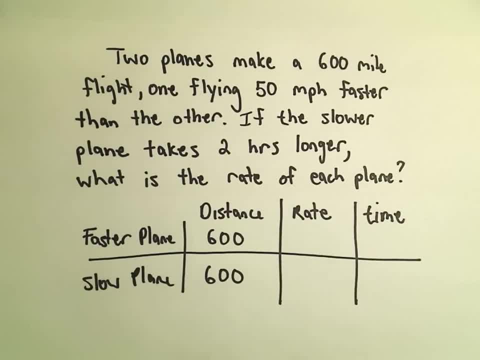 We don't know the rates, but so this is where we'll just start labeling things generically. The faster plane, its rate, let's just simply call it r, Since the faster plane is 50 miles per hour faster. that means the rate of the slow plane would have to be r minus 50.. 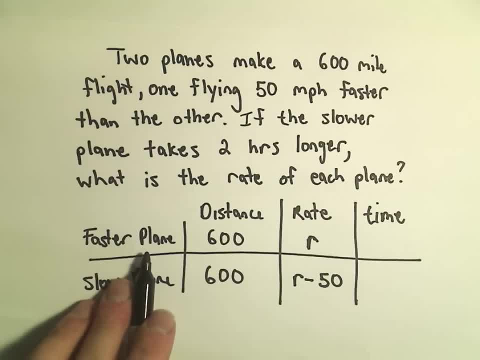 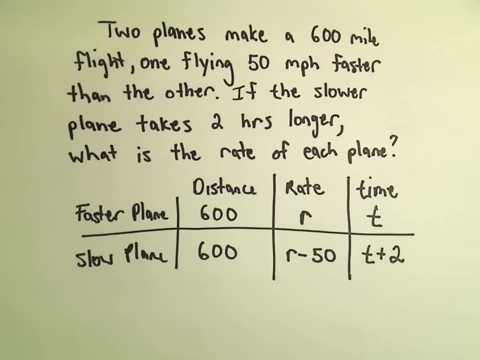 We can also likewise. we don't know the time it takes each, but suppose the faster plane takes t hours. Well, since the slower plane takes two extra hours, it would take t plus two hours to complete the journey. So now what we can do. we can use the fact that distance equals time. 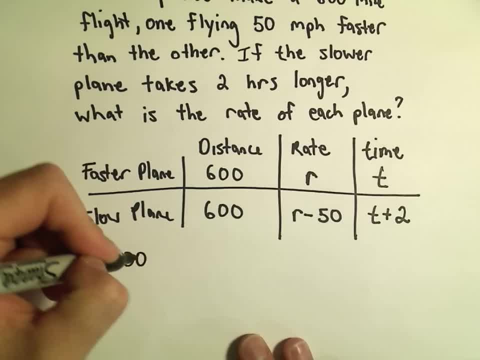 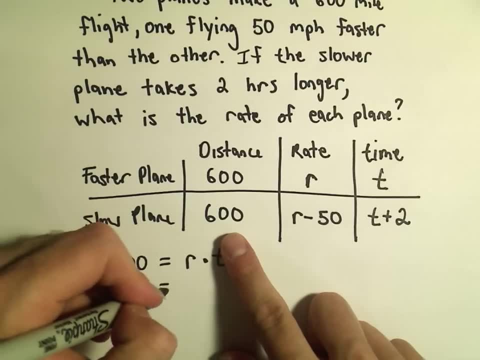 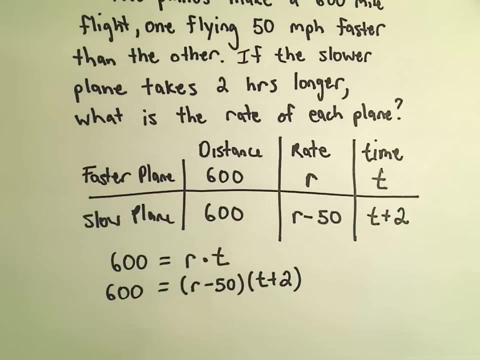 Distance equals rate times time. So for the fast plane we'll get 600 equals rate times time. And then for the slow plane we'll get 600 equals the rate which is r minus 50, times the time which is t plus two. 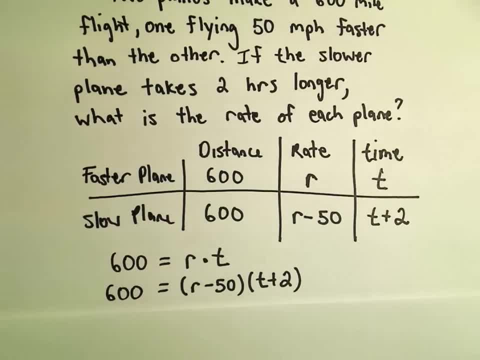 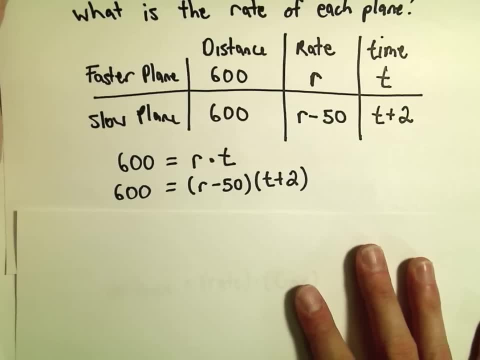 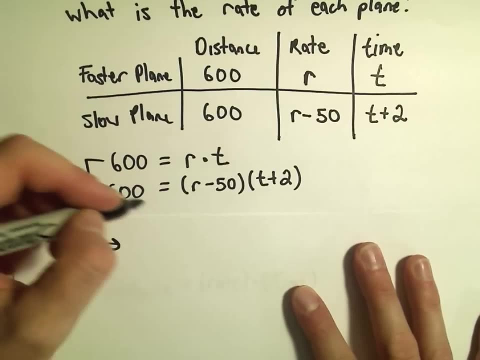 So now, what I'm going to do at this point is I'm going to take the first equation, Solve that for either t or r and plug that then into the second equation. So notice, if we take 600 equals r times t, If I divide both sides, let's say by r, I would get 600 over r equals t. 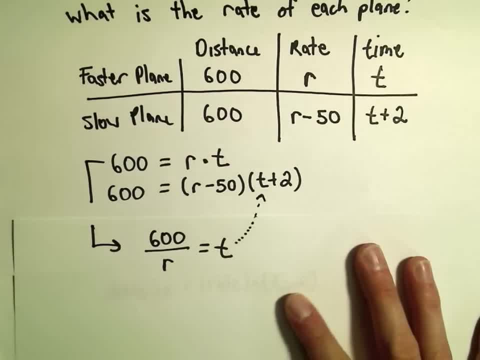 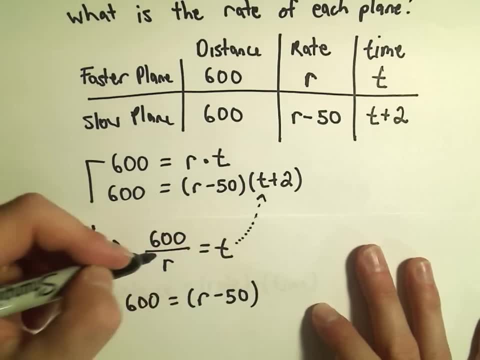 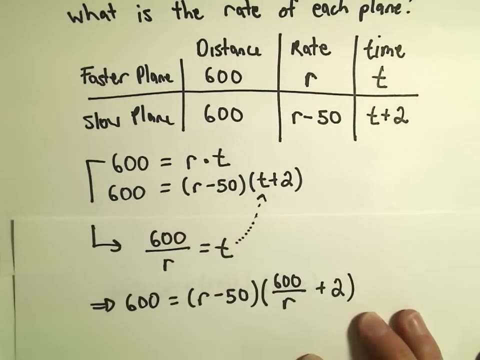 And what I'm going to do is I'm going to again just plug that into the second equation. So that tells me we have 600 equals r minus 50.. t in this case again, is 600.. Over r plus two. 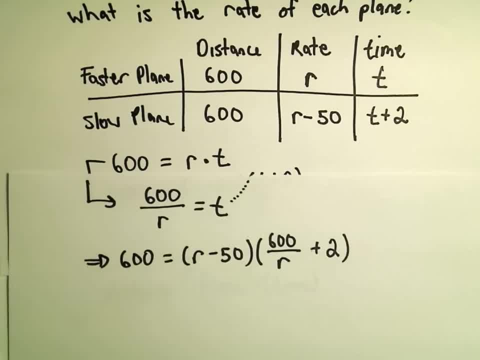 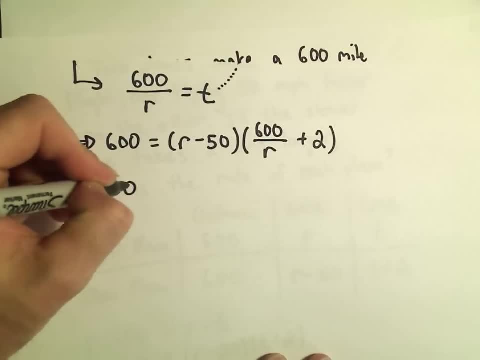 Okay, now there's a couple different ways we could go about simplifying this. I'm simply going to just go ahead and start distributing things on the right-hand side. So on the left we have 600 still just hanging out. r times 600 over r. 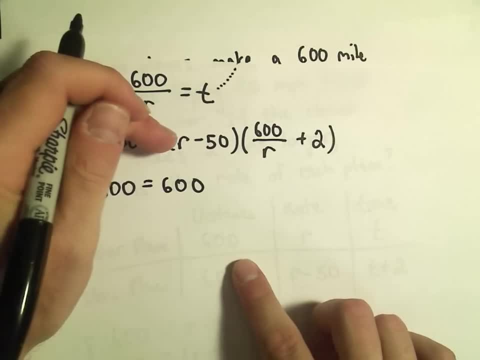 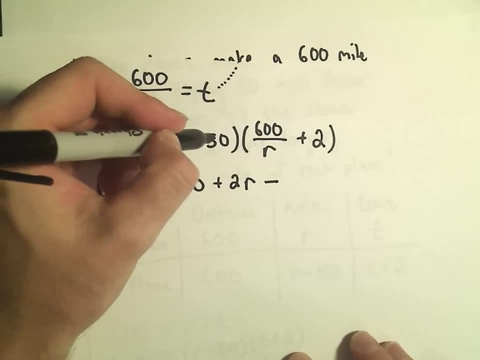 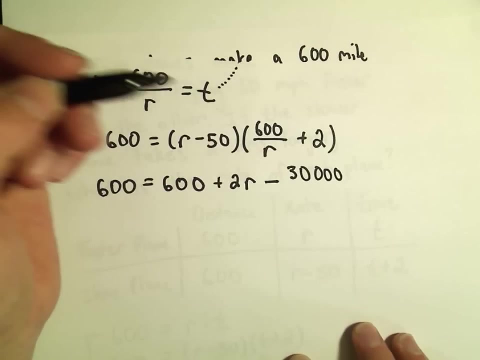 The r's would cancel, leaving us with just 600.. r times positive, two is positive, two r. We have a negative times a positive, That's a negative. Five times six is 30. And then we have an extra one, two, three. one, two, three zeros dividing by r. 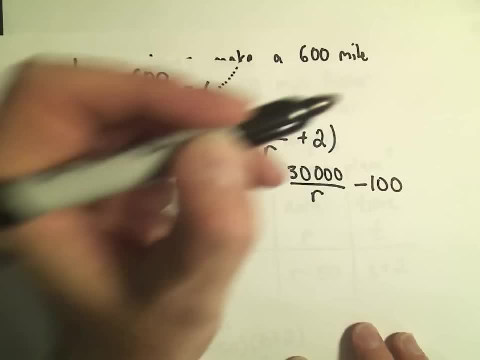 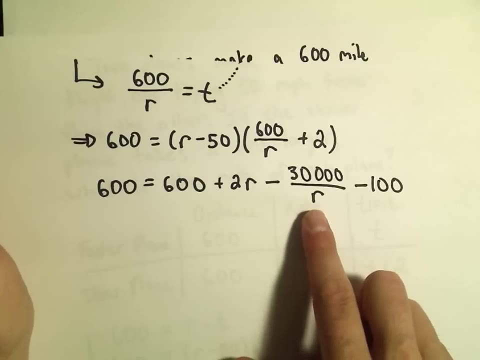 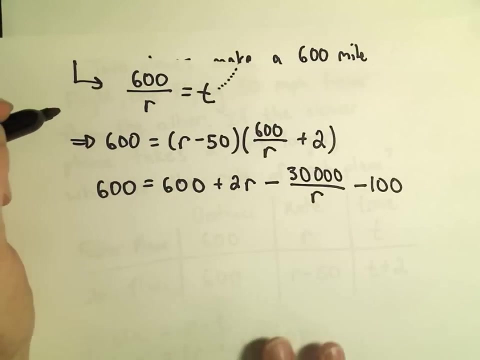 And then negative 50 times positive two is negative 100.. Okay, so I don't like a couple things. The main thing is I don't like this fraction on the right side. So everything else is being divided by just a one, except for this term that's being divided by r. 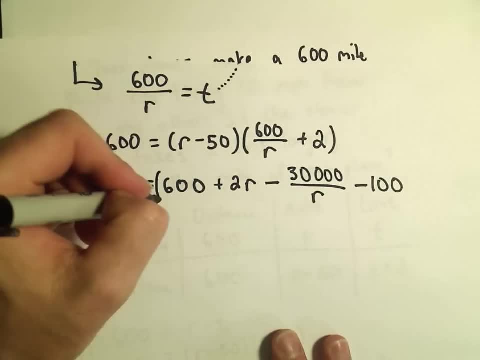 So to get rid of that, what I'm going to do is I'm going to multiply each side of my equation by r. Okay, so on the left side we would just have 600r. Now I have to distribute this r to everything. 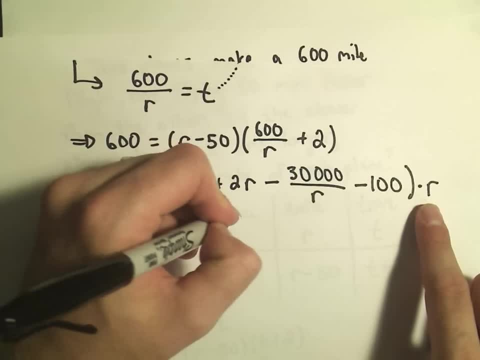 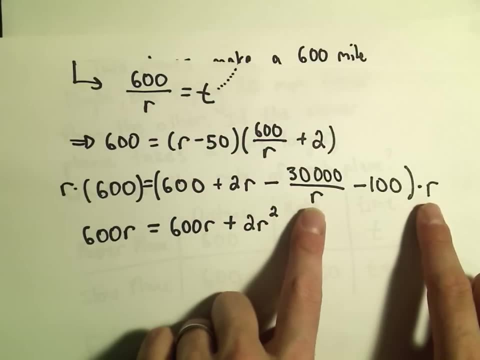 So again, we'll get another 600r. on the right side, We'll get two r times r, which is two r squared Negative 30,000 over r times r. The r's will cancel, leaving us with negative 30,000.. 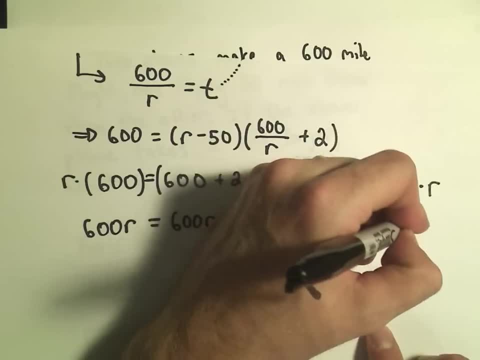 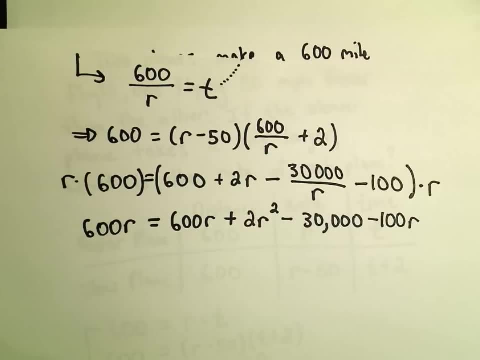 And then we'll get a negative 30,000 over r times r. Negative 100r. Okay, so finally, this is starting to look a little more like a normal quote-unquote quadratic equation to me. So again, we want to make one side zero. 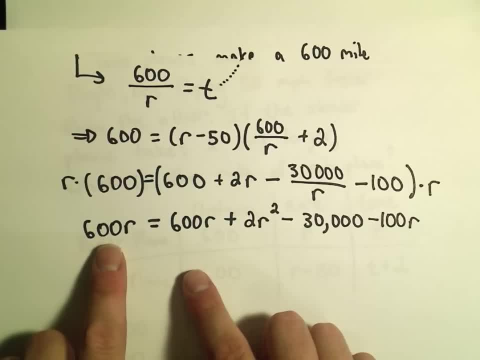 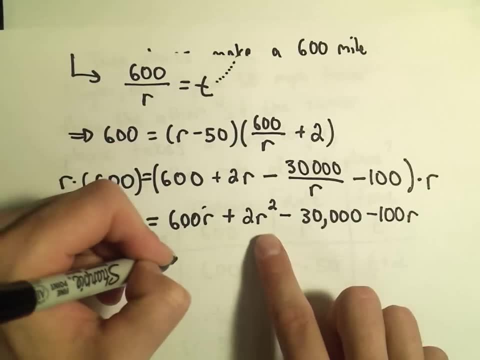 So we can do that by subtracting the 600r from the left side. If we do it to the right side as well, notice those would just cancel out. So we would have zero on the left, two r squared. I'm going to write the negative 100r in the middle. 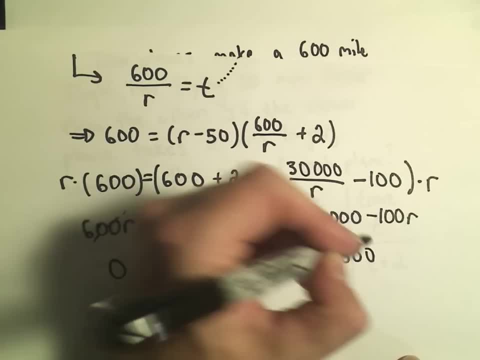 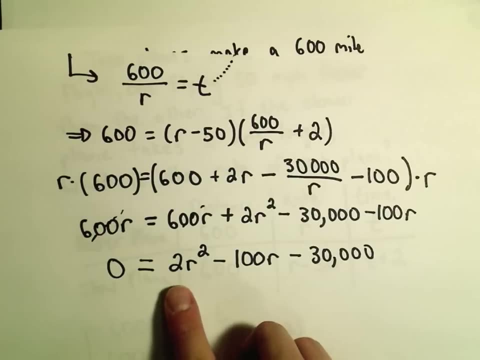 And then we've got this negative 30,000 also left over. So now I've got my quadratic. Again, I could use the quadratic formula. I'm going to try to factor, but first I'm going to divide both sides by two. 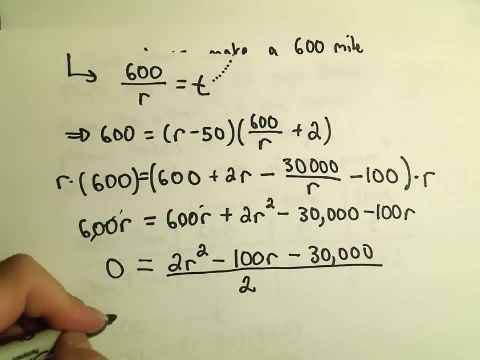 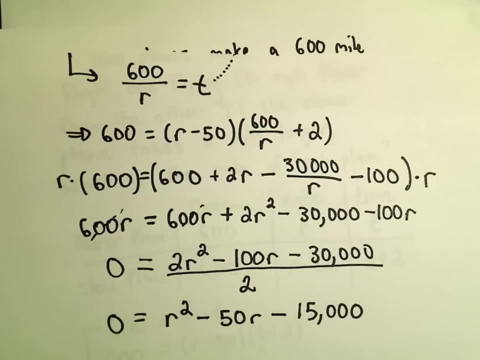 just to hopefully make the numbers a little bit easier to deal with. So two r squared over two is r squared Negative. 100 over two is negative 50r. And let's see 30 divided by two would be 15.. So I think negative 15,000 would be what we get. 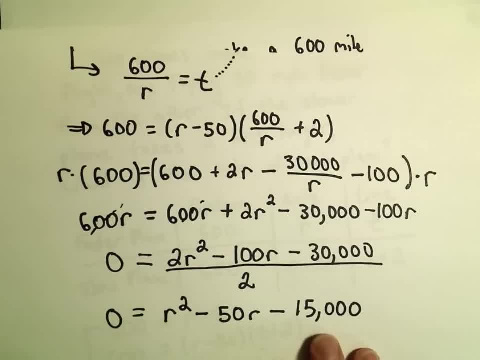 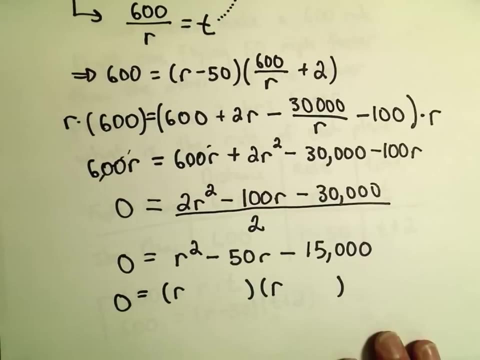 So okay, let's see if we can't think of two numbers that multiply to negative 15,000, but add up to negative 50. So again, you could use the quadratic formula if you're. you know, these numbers are definitely getting a little big.